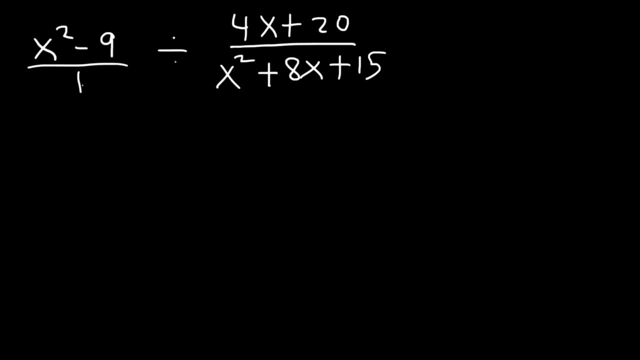 Now perhaps you've heard of the expression keep, change, flip. Well, here's how you use it: Keep the first fraction the same, So let's rewrite it And then change division to multiplication And then flip the second fraction. And now all we need to do is factor and cancel. 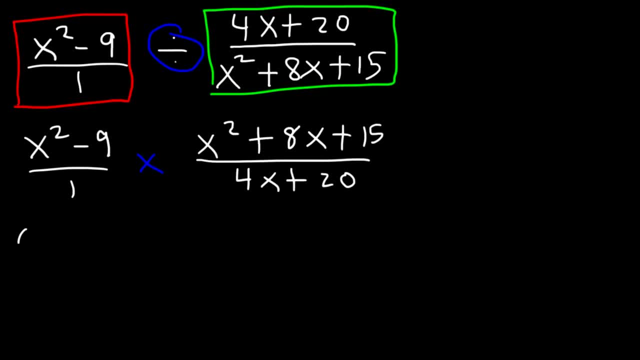 x squared minus 9.. We can factor as x plus 3 times x minus 3.. x squared plus 8x plus 15.. Two numbers that multiply to 15 but add to 8 are 3 and 5.. So it's going to be x plus 3 times x plus 5.. 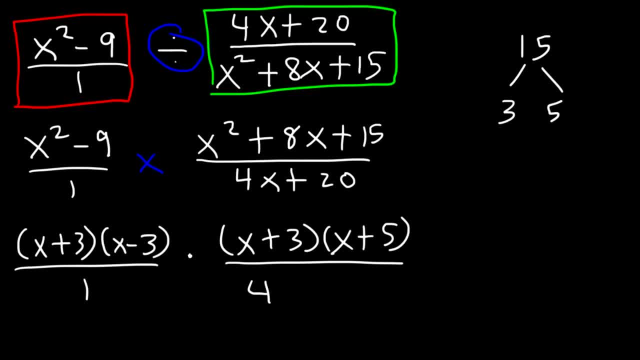 Now 4x plus 20.. We can take out the GCF, which is 4. And that's going to leave us with x plus 3 times x plus 5.. Now we want to determine the excluded values. The excluded value is negative, 5.. 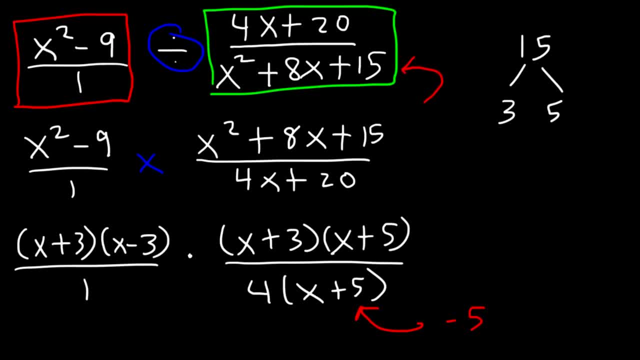 You can see that here. But also this is in the bottom of a fraction, So which is x plus 3 and x plus 5.. So negative 3 and negative 5, which correlates to this part, while it's in the bottom of a fraction. those are excluded values too. 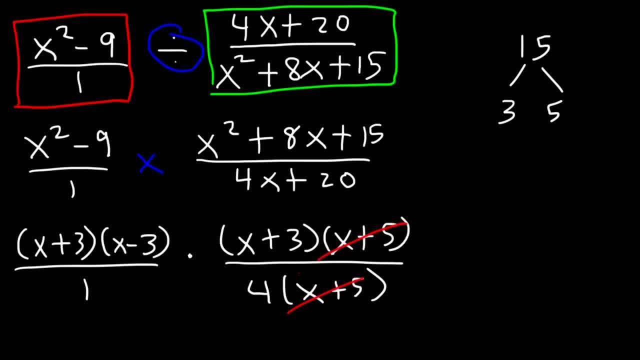 Now let's cancel. The only thing that we can cancel is x plus 5.. And these two we can write it as x plus 3 squared times the other one, x minus 3, divided by 4.. So that's the final answer for this problem. 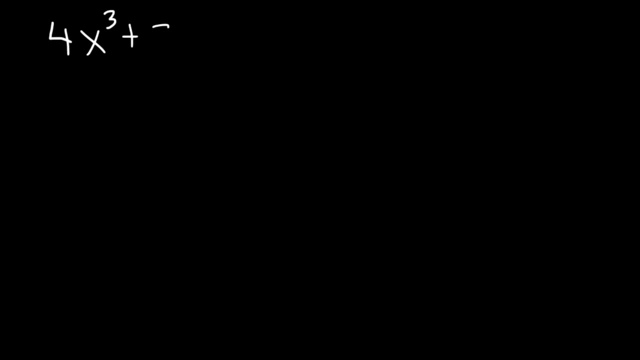 Let's try this one: 4x cubed plus 32.. Divided by 6x squared minus 24.. Divided by 3x squared minus 6x plus 12.. Over x squared minus 7x plus 10.. 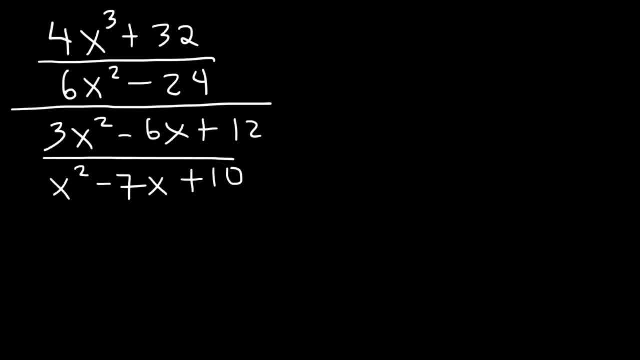 So how can we simplify this complex fraction? If you ever see a problem like this, you can rewrite it. This is equivalent to 4x cubed plus 32 over 6x squared minus 24.. Divided by whenever you see a fraction, it represents division. 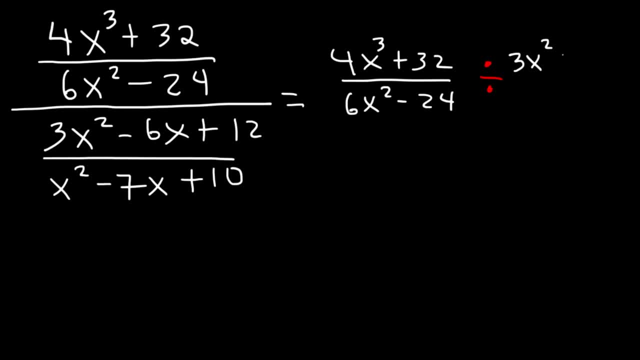 So we're going to divide it by the other stuff: 3x squared minus 6x plus 12.. Okay, that's a terrible 2.. Over x squared minus 7x plus 10.. So now that we're dividing these rational expressions, let's use the keep-change-flip technique. 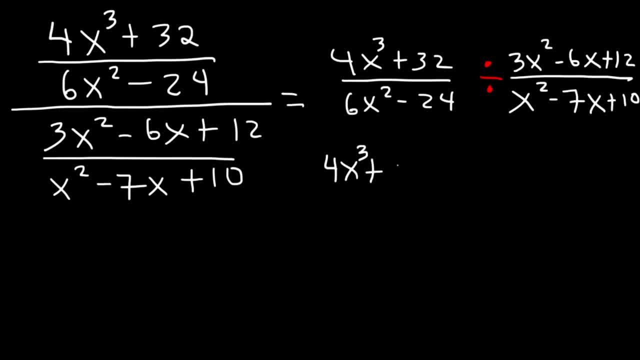 So let's keep the first part the same And then let's change division to multiplication, Okay, And let's flip the second fraction. Now let's factor and cancel, So 4x cubed plus 32.. The first thing that we can do right now is take out a 4.. 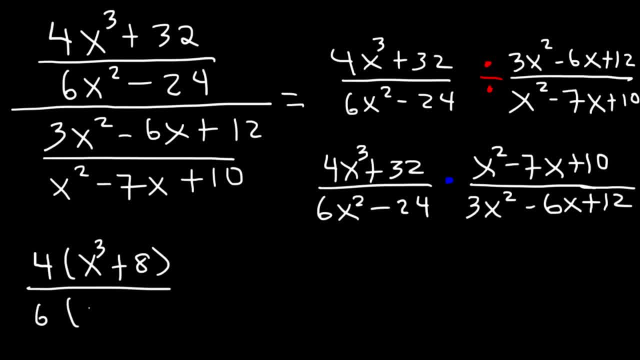 And 6x squared minus 24, we can take out the GCF, which is 6.. Now x squared minus 7x plus 10.. Two numbers that multiply to 10 but add to negative 7 are negative 5 and negative 2.. 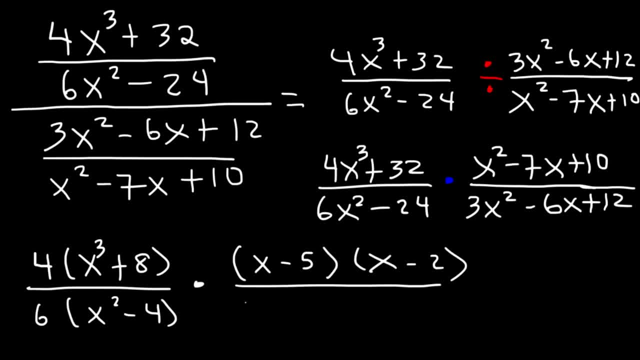 And for the other one, we can take out the greatest common factor, which is 3.. And that's going to leave behind x squared minus 2x, And 12 divided by 3 is 4.. So now, how can we factor x cubed plus 8?? 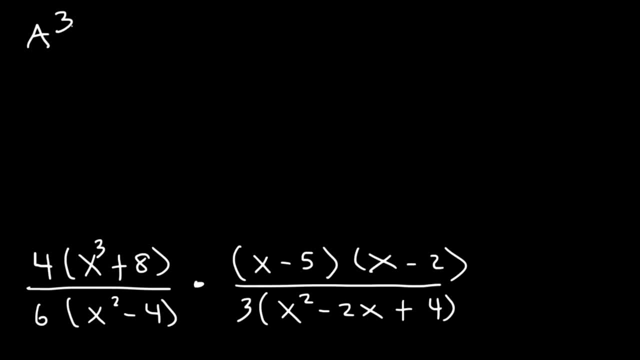 Notice that we have the same number of numbers, So we can use this formula: a cubed plus b cubed is a plus b times a squared minus ab plus b squared. So x cubed is a cubed, b cubed is 8, which means that a is x, b is 2.. 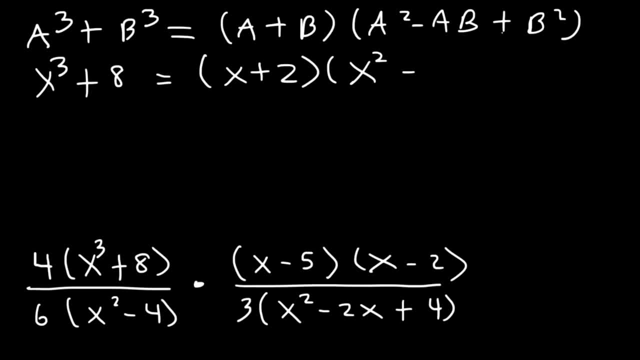 a squared x times x, that's x squared ab. x times 2, is 2x. b squared 2 squared is 4.. And so that's what we have. So this is going to be 4 times x plus 2 times x, squared minus 2x plus 4.. 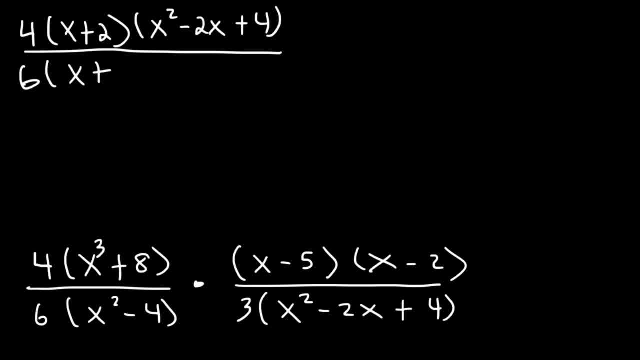 And x squared minus 4, that's x plus 2 times x minus 2.. Now it turns out that we cannot factor x squared minus 2x plus 4.. So we just have to leave it the way it is. Now let's cancel. 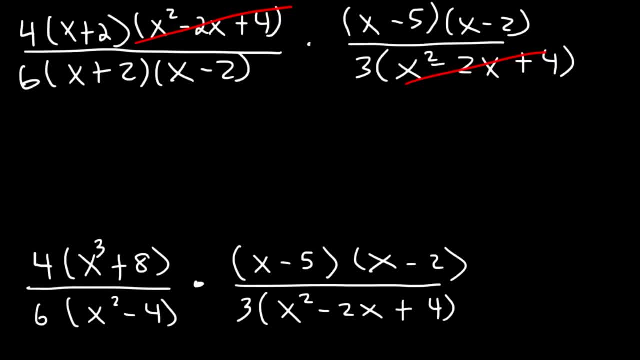 We can cancel those two. We can get rid of x plus 2.. And also x minus 2.. 4 over 6 can be reduced to 2 over 3. And we have this other 3 as well. So the final answer is 2 times x minus 5, divided by 9.. 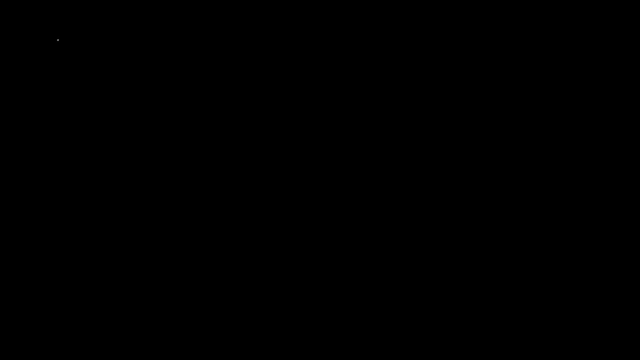 That's it. So let's say, if we have the polynomial 8x cubed minus 4x, squared plus 12x, A polynomial is simply an expression with many terms And we're going to divide it by a monomial or one term. 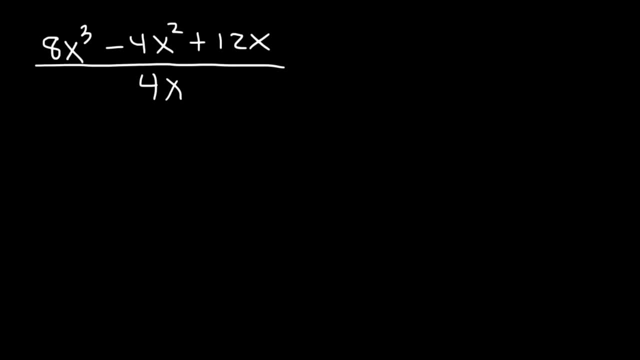 Whenever you want to divide it by a monomial, you can separate this fraction into three separate fractions. So basically, you want to divide every term on top by 4x 8x. cubed divided by 4x 8 divided by 4 is 2.. 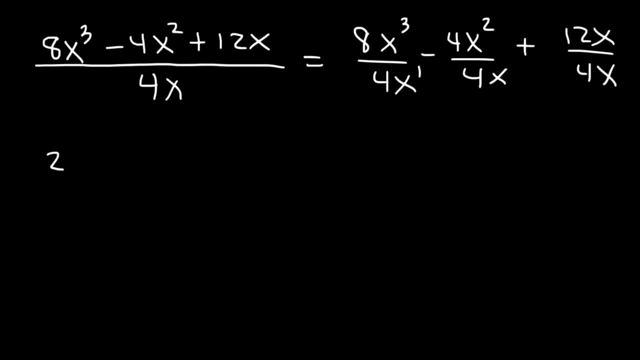 x cubed divided by x is going to be x squared. You've got to subtract the x points. 3 minus 1 is 2.. So this is going to be 2x squared Negative. 4x squared divided by 4x is simply negative x. 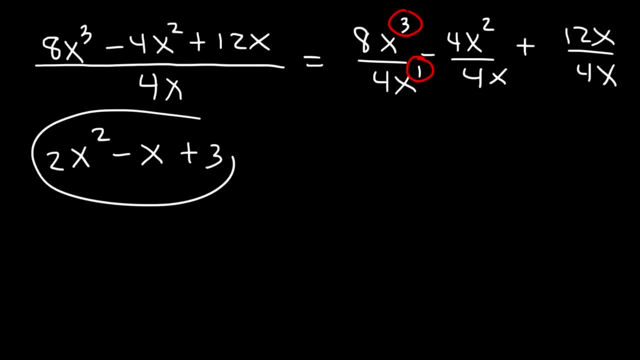 And 12x divided by 4 is 3.. So that's the answer: 2x squared minus x plus 3.. Let's try one more example: 36x to the 5th minus 63x to the 4th. 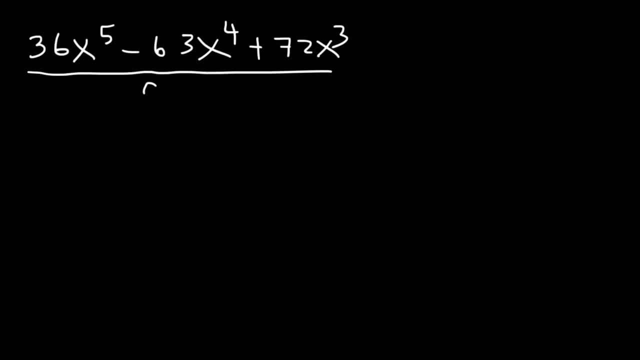 Plus 72x cubed Divided by 9x squared. Feel free to try this example. So let's divide every term by 9x squared. So 36 divided by 9 is 4. And 5 minus 2 is 3.. 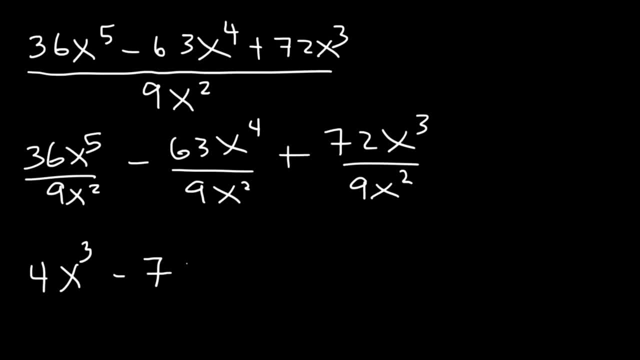 63 divided by 9 is 7.. 4 minus 2 is 2.. 72 divided by 9 is 8.. 3 minus 2 is 1.. So the answer is 4x cubed minus 7x, squared plus 8x. 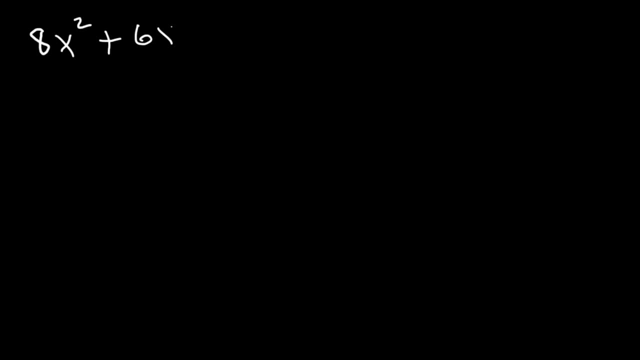 Let's say if we have 8x squared plus 6x minus 12.. And let's divide it by 2x minus 3.. Now we can't separate it into smaller fractions. I mean we could, but it's going to be pointless. 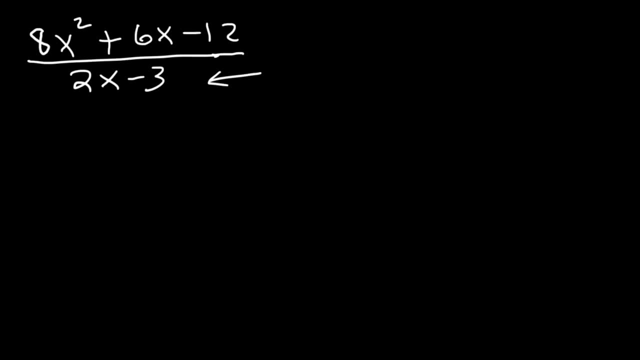 If you have two or more terms in the bottom, you want to use long division, The numerator is going to go on the inside. Actually, I might need a little bit more space, So let's put this here And now. let's divide. 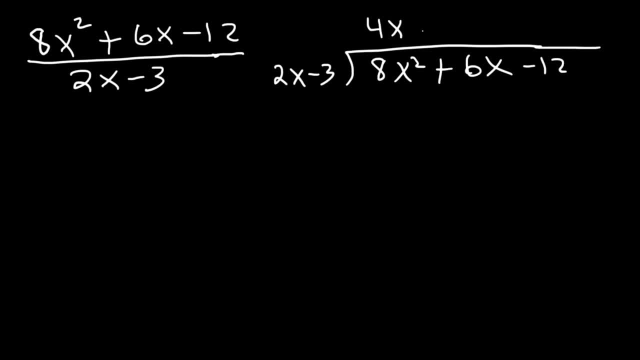 8x squared, divided by 2x is 4x. And now let's multiply: 4x times 2x is going to be 8x squared, And 4x times negative. 3 is negative 12x, And then subtract. 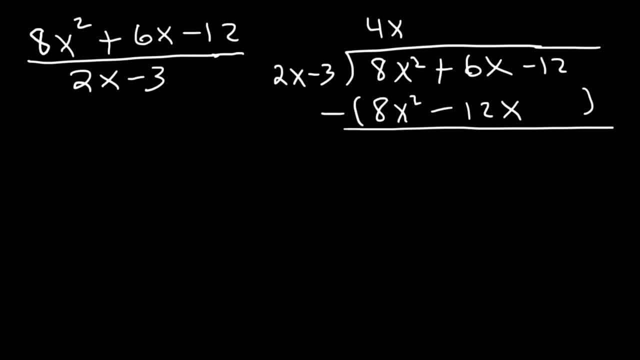 So you're always going to repeat the process: Divide, multiply and then subtract. 8x squared minus 8x squared is 0.. 6x minus negative 12x, That's the same as 6x plus 12x. 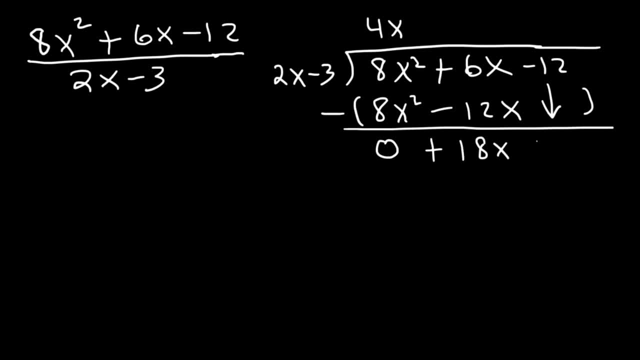 That's positive 18x, And then bring down the negative 12.. Now let's divide again. 18x divided by 2x is 9.. And then subtract. Well, first we're going to multiply: 9 times 2x is 18x. 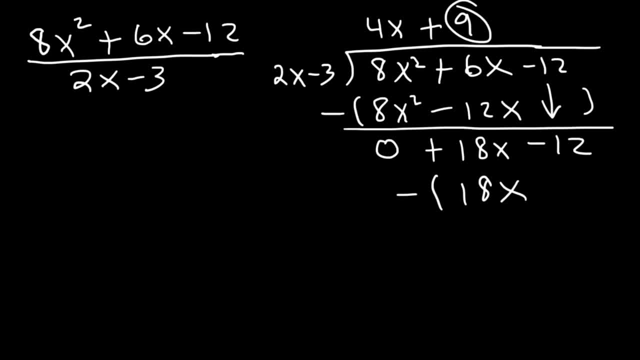 And 9 times 9x is 9x, And 9 times 9x is negative. 3 is negative 27.. Now we can subtract 18x minus 18x. That's going to be 0.. Negative: 12 minus negative 12.. 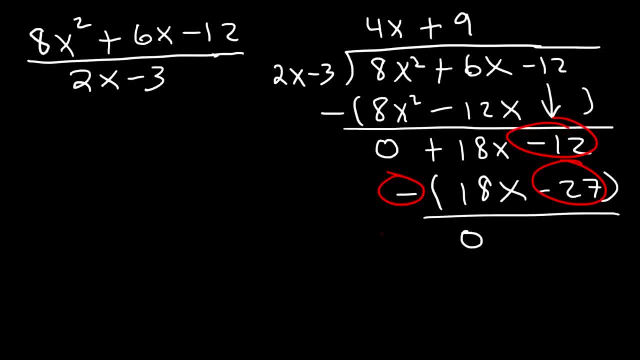 I mean minus negative 27. That's the same as negative 12 plus 27. Which is positive 15. And positive 15 is the remainder. So now the answer: 8x squared plus 6x minus 12, divided by 2x minus 3. 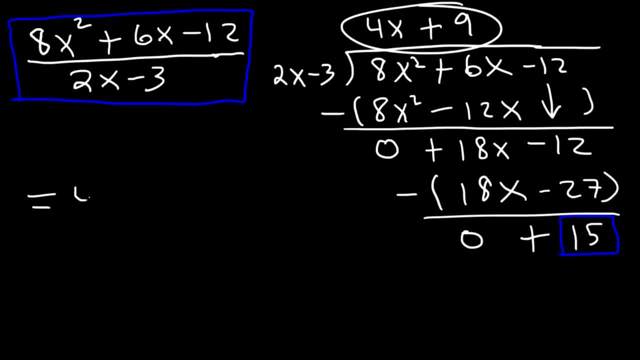 is equal to the stuff that you see on top, Which is 4x plus 9.. And then plus the remainder divided by what you tried to divide it by, which is 2x minus 3.. So that's the solution to the problem. 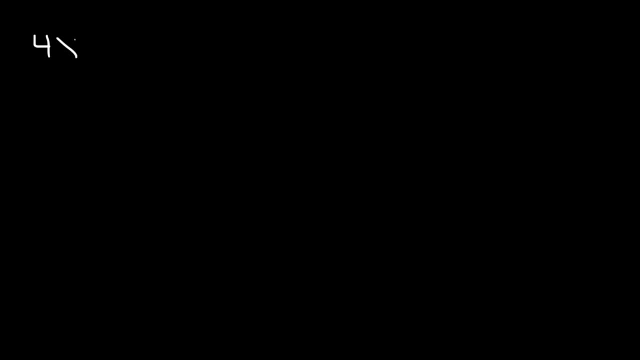 Now let's work on another example. Let's divide 4x cubed plus 10x minus 8 by x minus 2.. So feel free to pause the video and work on this example. So let's put the denominator on the outside and the numerator on the inside. 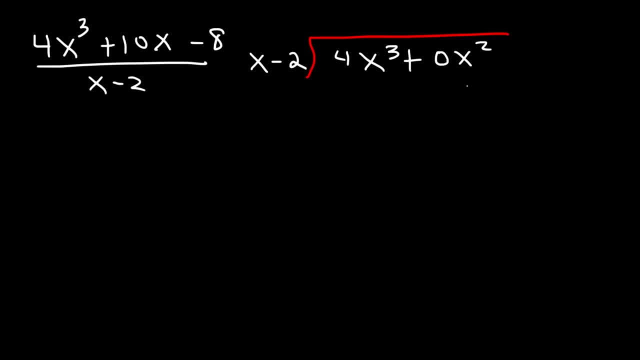 Now we need to write this as 4x cubed plus 0x squared. If you don't see an x squared, add 0x squared Plus 10x minus 8.. So let's divide 4x cubed. divided by x is 4x squared. 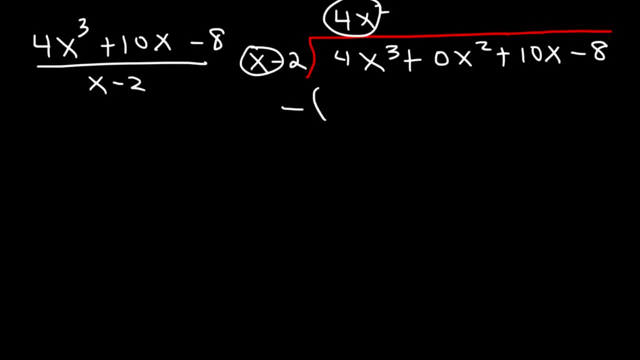 And now let's multiply 4x squared times x, that's 4x cubed. 4x squared times negative 2, that's going to be negative 8x squared. Now we can subtract 4x cubed minus 4x cubed is 0.. 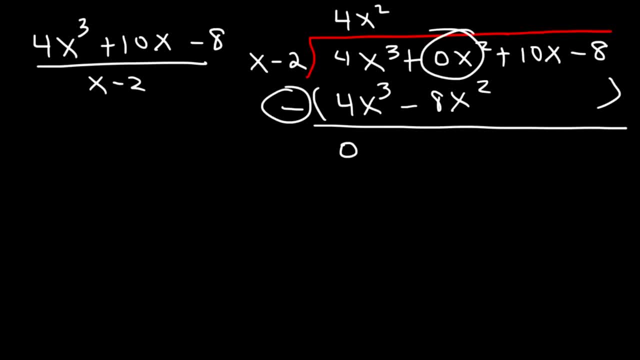 0x squared minus negative x squared is basically 0 plus 8.. So that's going to be positive 8x squared. Next, let's bring down the 10x. Now let's divide 8x squared by x, So that's going to be positive.